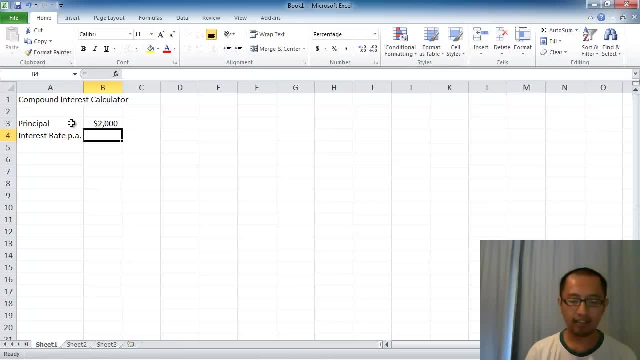 with saving two thousand dollars in the bank at interests rate of five thousand dollars. Look at that. que78a percent per annum. okay, now we're gonna put this information into the spreadsheet. so in cell b6 I'm gonna put in the year. okay, so we have year one. 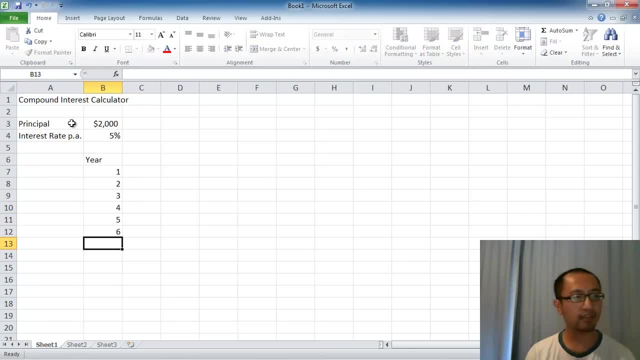 year two, year three, year four and so on. okay, then we have the principal at the beginning of the year. so how much money you have in the bank at the beginning of the year? initially we start with the $2,000. okay, so I just pressed equals and 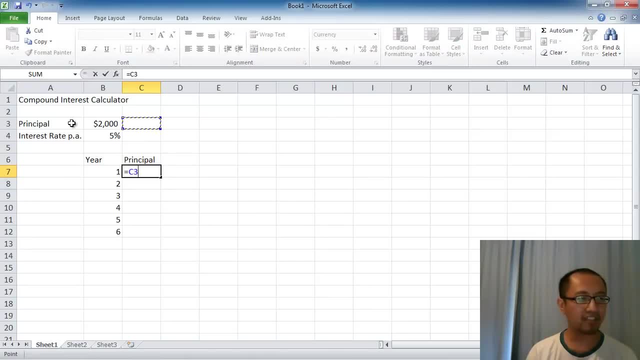 I move, I use the arrow keys to move the box to cell b3 and I press ENTER. so now this cell refers to cell b3. so whatever number that I update in cell b3- so for example, if I changes to two thousand three hundred, it'll automatically update cell c7 as well. okay, and then the next thing I do: 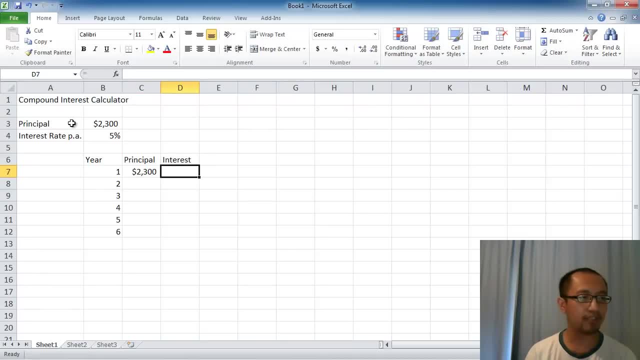 is I calculate how much interest I earn during that year. so what I'm gonna do is I'm gonna equal the principal at the beginning of the year, times by the interest rate, which is 5%. so that year I'm going to earn a hundred and fifteen. 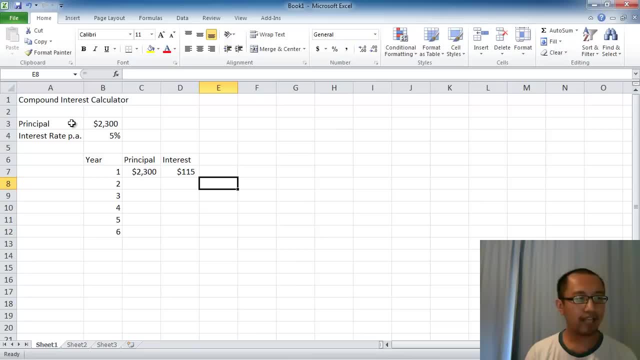 dollars and then what's going to happen is, at the end of the year, how much principal I have, end of year principal and that's going to be my principal at the beginning of the year, plus the interest that I'm earning. okay, so this year, originally I 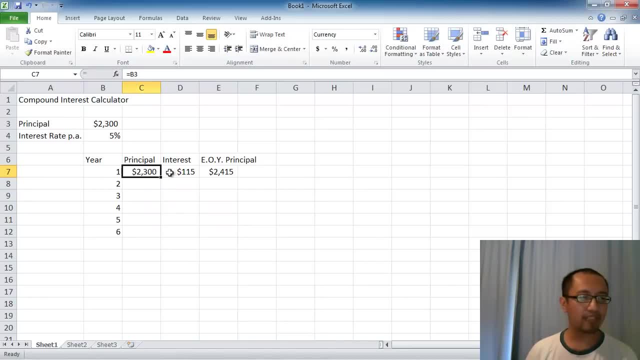 had two thousand three hundred dollars. I added on five percent, which is a hundred and fifteen dollars, and I ended up with two thousand four hundred and fifty. okay, and then in the second year I will start with the principal that I have at the end of the first year. so I press equals. 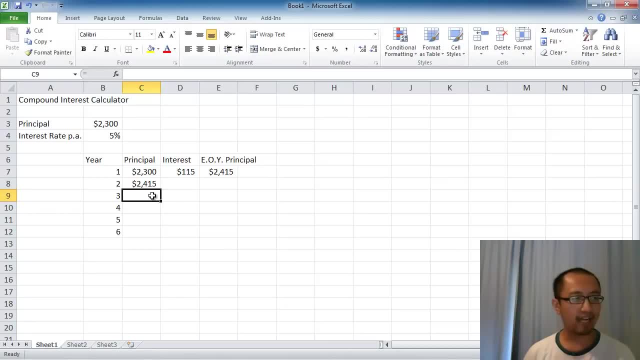 e7 and now that's the principal I have. at the beginning of year two the interest that I earn will be equal to the principal at the beginning of the second year, times by the interest rate, which is B4, and then the end of year principal will equal the principal. 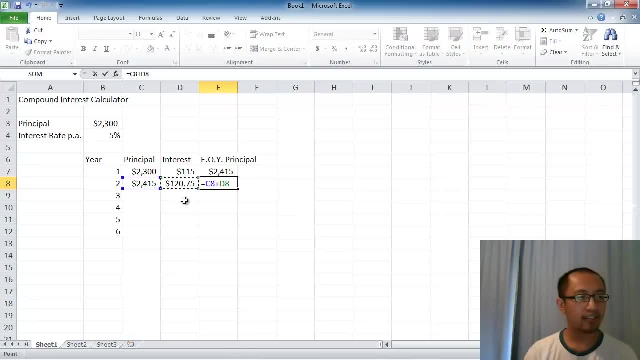 at the beginning of the year, plus the interest, and it's $2,535.. Now you must be asking the question: well, do I have to keep entering this every single line? and the answer is no. you don't have to keep doing that. all you have to do is you can highlight these three. 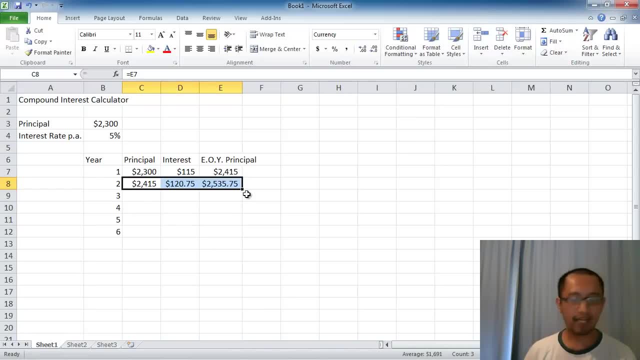 cells and you can see that there is a black solid dot at the bottom right hand corner and all you have to do is drag that dot down and you can see it automatically fills all the cells. Now here is a big problem. you can see here that an error has occurred and that's because 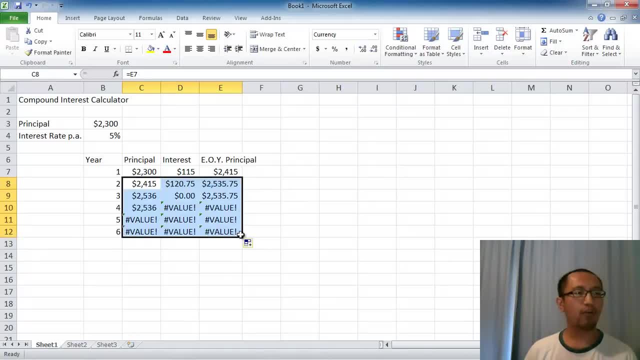 when you select some cells and you fill down, what Excel does is it looks at the formula that you have entered in the cells and you can see here I have E7. so what Excel does when you fill down is Excel keeps the letter the same. so E will still be there, but it will. 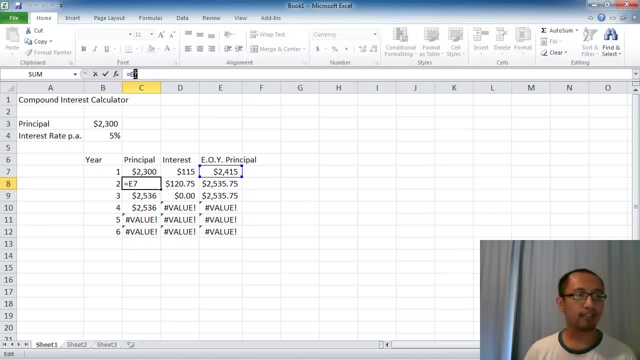 increase that number by one every row. so you can see here in the next box it says E8 and we have E9. So that part is okay because our principal at the beginning of the year is going to equal the principal at the end of the previous year. so that is okay. but if we look at the interest, 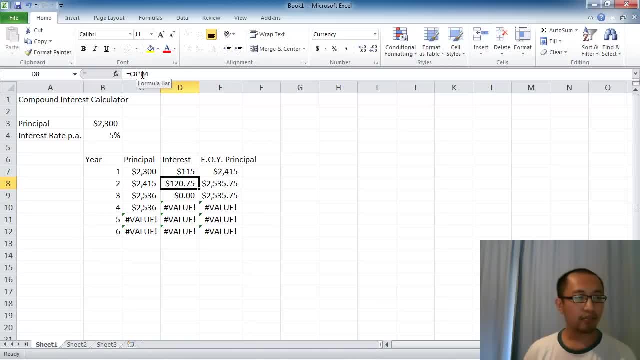 so when we fill down Here I am originally doing the principal, which is C8 multiplied by the interest, which is B4. so that is okay. but when you fill down it's turned into C9 times by B5. now there is nothing in B5, so we want to change this B4 somehow. so Excel knows that when we fill down 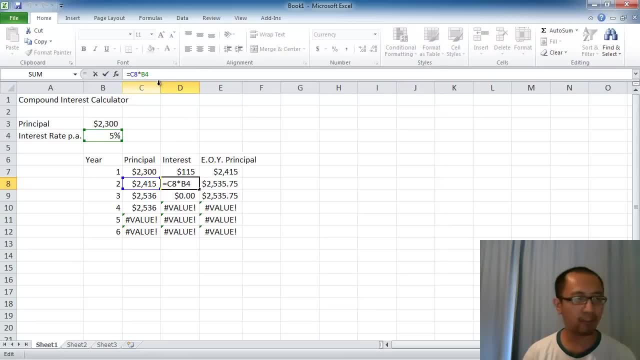 we don't want it to change the number 4.. We want to make the number 4 stable. So I am going to lock it to that cell by putting a dollar sign in front of the number 4 and then when you fill down. 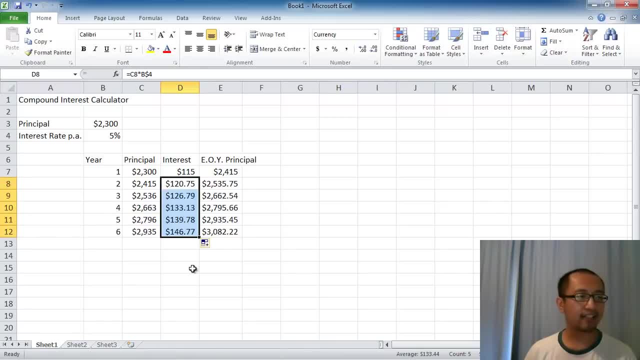 So I am going to fill down and you can see that all the errors are fixed, because now every formula is now referring to this box. so it is the principal multiplied by the interest rate in this box. Okay, so It is now working as well. so that is what the dollar sign refers to. it refers to absolute. 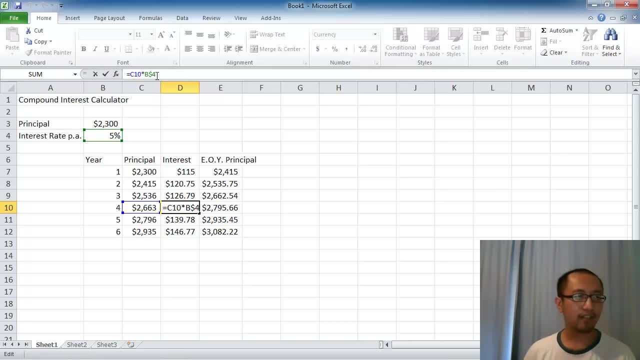 referencing. okay, which means that we don't adjust the formula when we are filling down. Okay, now let's look at the end of year principal. so we are just getting the principal from the beginning of the year, plus the interest gives you the end of year principal. 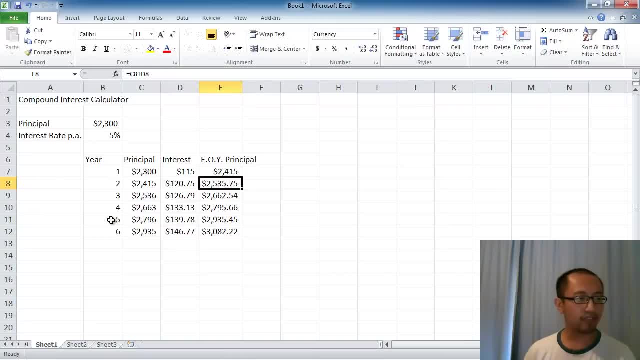 So, once you have filled down a few cells, what I am going to do Is I highlight the bottom two cells and I just keep filling down, because Excel now has an idea of what I am trying to do. so I can fill down to 25 years and you can see here. 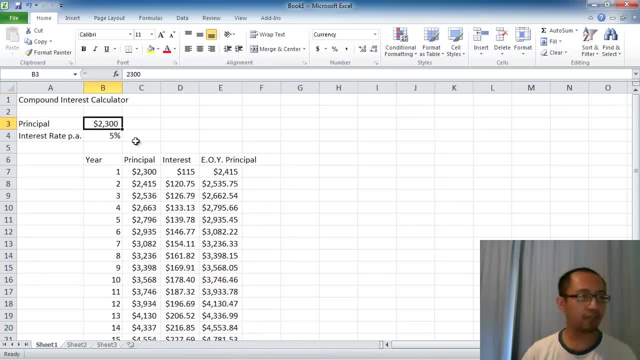 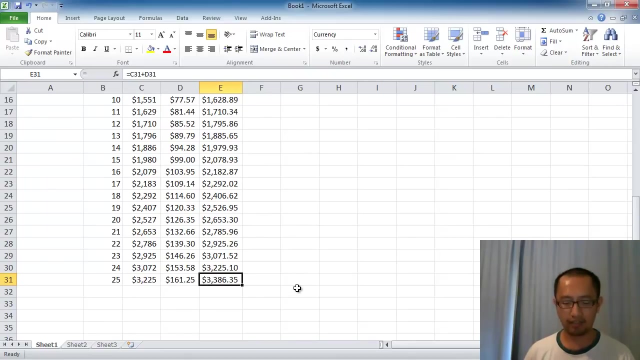 approximately, if I save okay, instead of 2300, I am just going to save a thousand dollars, so you can see the impact. so if I save a thousand dollars and the bank gives me 5% interest per year, Then what is going to happen at the end of 25 years is I will end up with 3386 dollars. 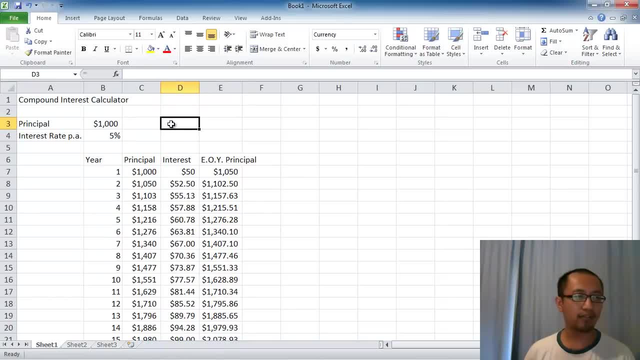 Okay, so for those of us that understand the maths quite well, this interest rate is compounded yearly. okay, if you want to do a monthly interest rate, you will have to change this to months and then you will have to make other adjustments. But right now this is an interest calculator based on the fact that the interest rate is. 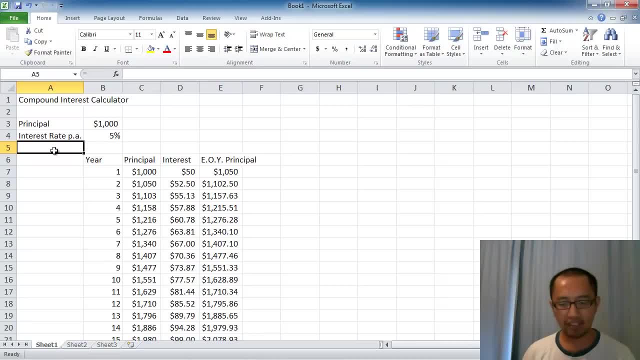 compounded yearly. Okay, thanks for watching guys. see you next time.